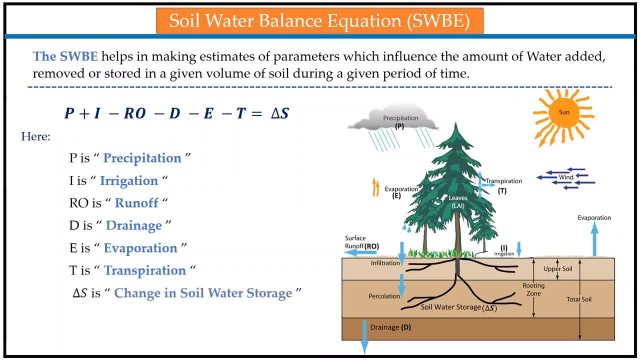 from the soil. finally, we are able to get the change in soil water storage using all the parameters from out. of all these, precipitation and irrigation are the one that add water to the soil and rest for that. we are able to see runoff, drainage, evaporation and transpiration. these are the factors that are responsible for. 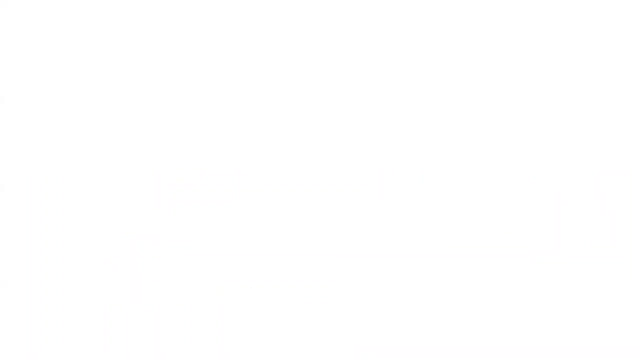 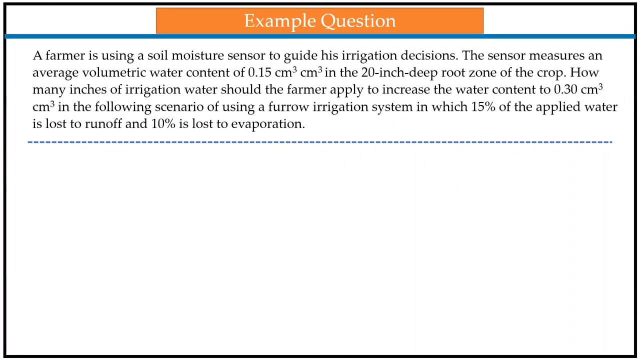 decrease in soil water for the moving ahead. here is an example question which is used to in which soil water balance equation is used. so here is a farmer is using, who is using soil moisture sensors to guide his irrigation decisions. so he has to decide how much of irrigation he have to give to his field. the parameters: 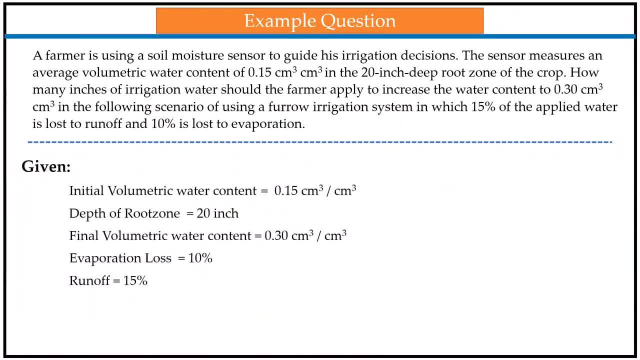 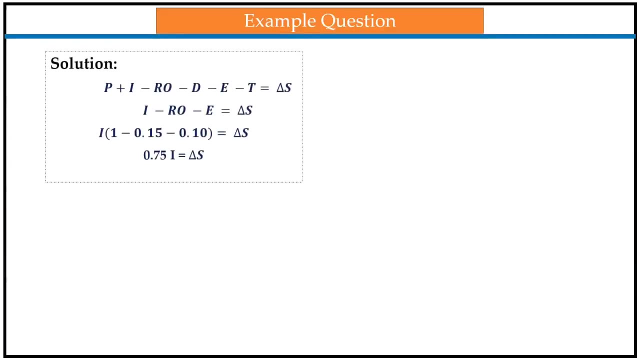 are the amounts. the values that are given to us are initial volumetric water content and the depth of the root zone, final volumetric water content, the losses due to evaporation and the loss of water due to runoff. so what we have to find is amount of irrigation that we have to apply to the field. moving ahead here is: 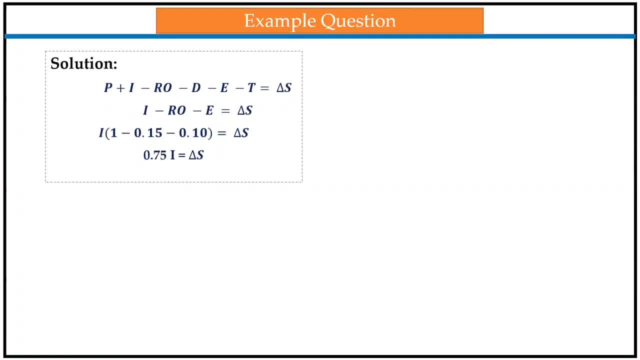 the solution and this first step of the solution. we are using the main soil water balance equation. over here we are able to see all the parameters that are contributing to that. this equation, as a result we arrive at so with this, simplement losses. this equation we've been trying to solve above is going by comparison on a. 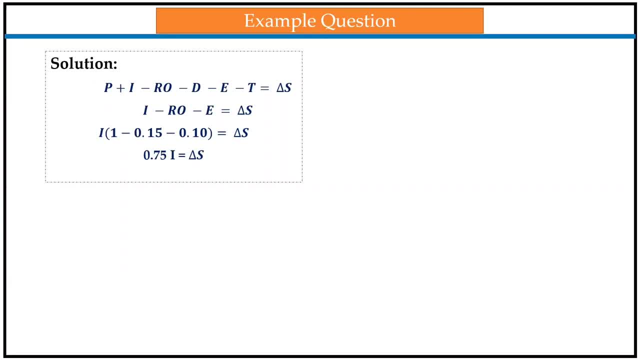 100 percent of losses are federated to the reformingDSO. since wave of 5 Temperature change up is 15%, loses are about 13% loss or 10%. this jump damage in-between 5.1 and 6 yards. we have milk, Little Potent importer sources and this change Anthro twist a little bit slipped into the soil to control the. 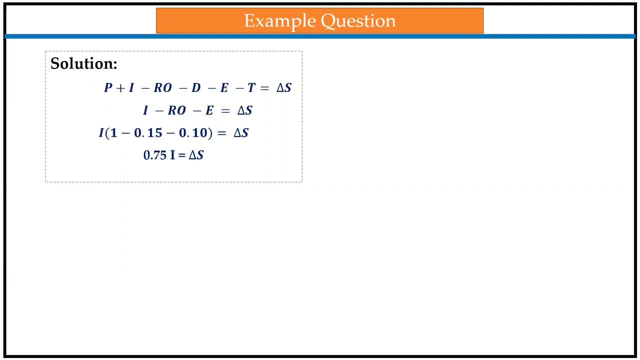 soil, while the other soil are femtosecond layer. so these families may have lost 14% hit and trial and we'll be able to get the irrigation in comparison to change in soil water storage further. moving on to the second step, we were given final volumetric water content and the initial volumetric water content, along with 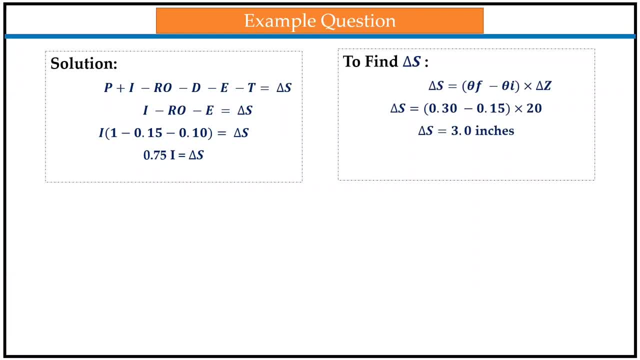 it was the depth of root zone. so by solving this equation we'll be able to find the change in soil water storage. that is, we get an answer of three inches. and further, taking both these solutions of the first step and the second step, when we compare them both, we'll be able to get: